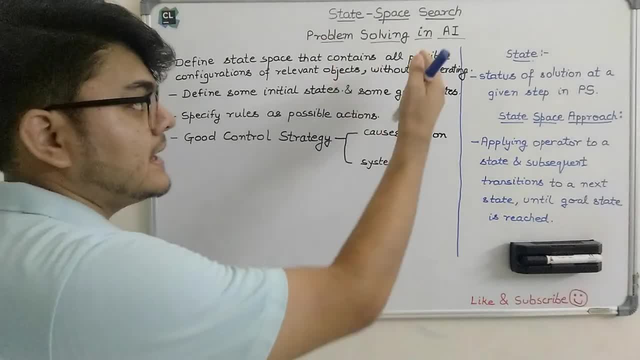 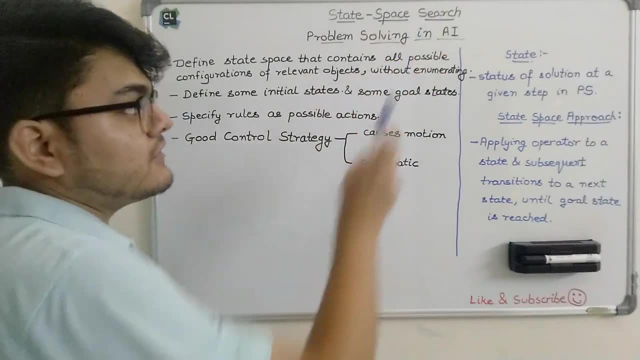 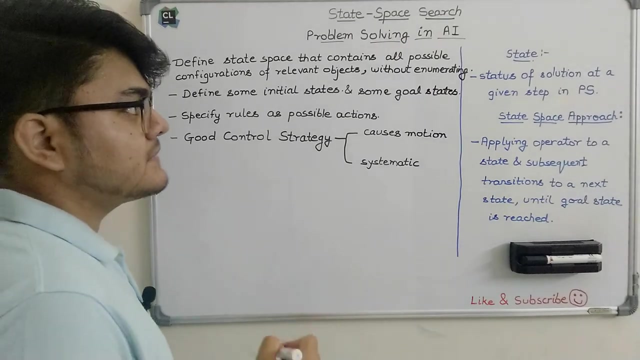 basically, we are trying. what we're trying to do is we're trying to implement problem solving in AI using this state space search technique. Now, before moving on to this technique, I just want to give a very ah, simple problem, which is also known as the monkey banana problem. 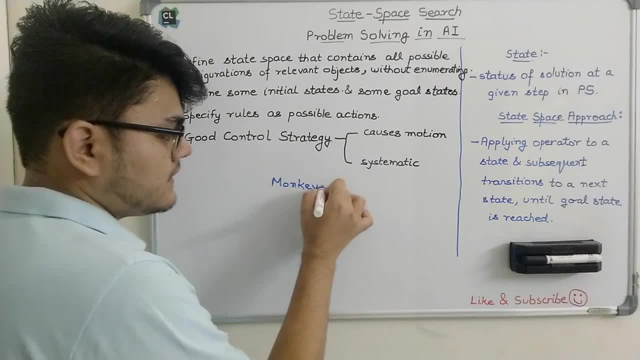 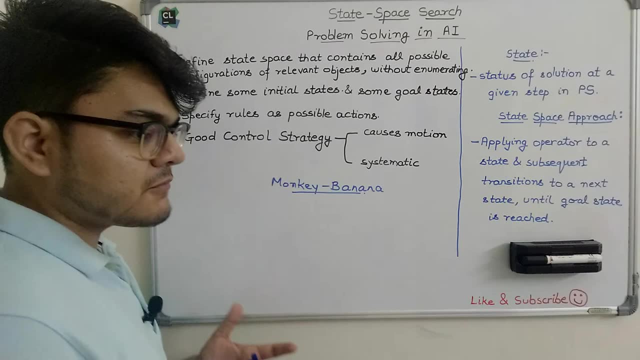 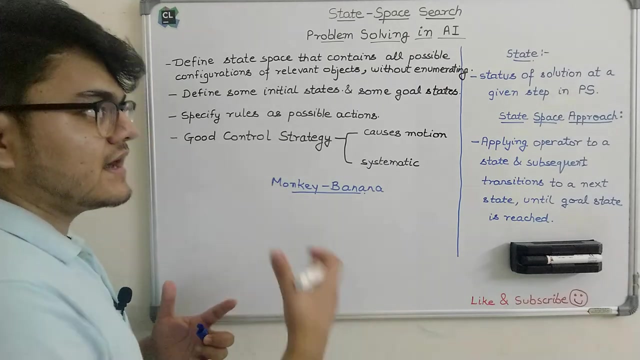 They're the monkey-banana problem. right, It is a monkey-banana problem. It is a very simple problem for humans to solve, but you will see that in prologue we can actually implement that and an artificial intelligence program will be able to solve of this. 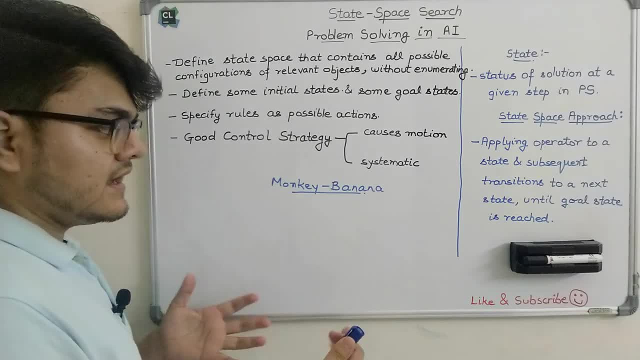 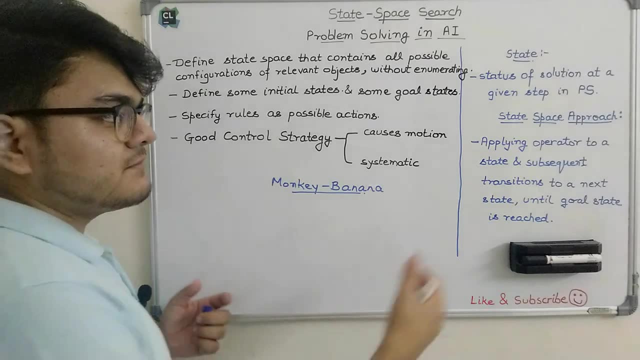 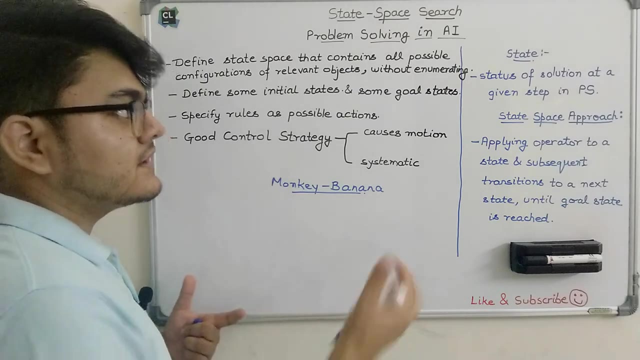 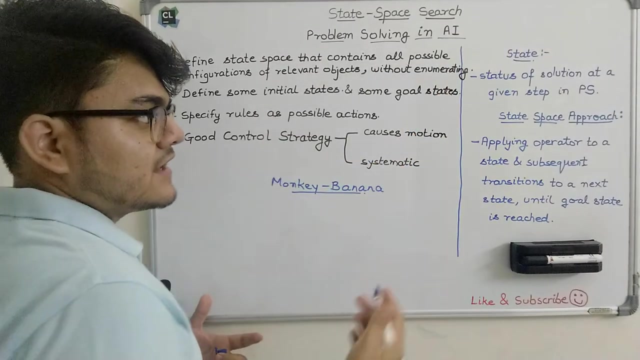 problem, and it really looks very great how AI can solve the real-life problems. So let me just give you a quick overview of this problem, because before understanding these definitions, we will first have to understand why problem solving is required, right? So what are the types of problems that an artificial intelligent agent can use? 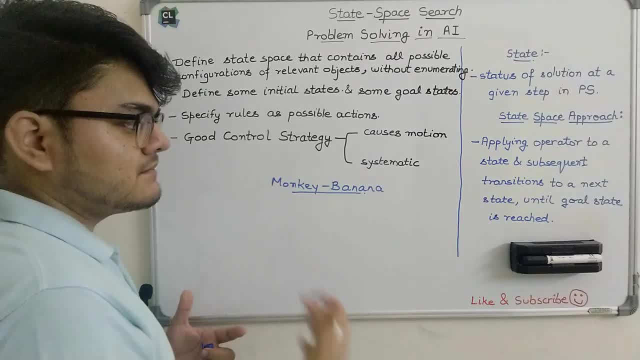 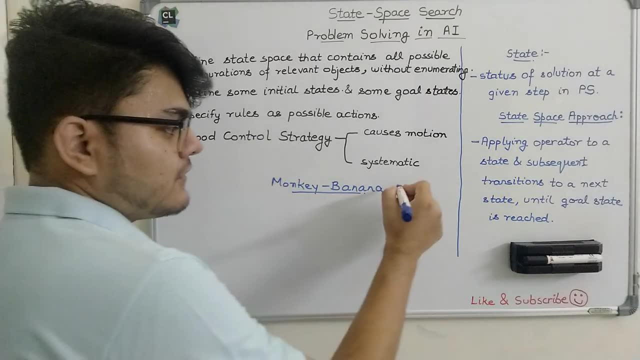 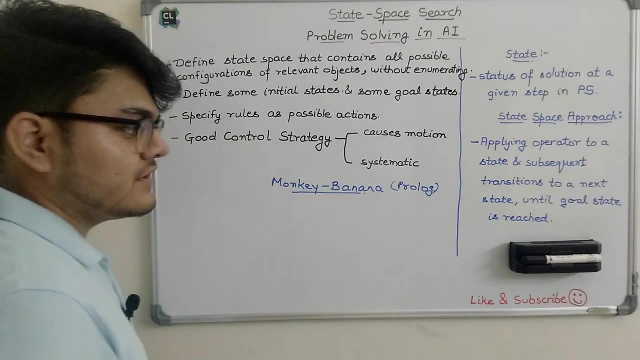 So we will first have to make sure- or I'm just making this sure- that you will understand some of the very good examples that I'm going to show here, And we will also implement this problem in Prolog, which is actually logical programming language, right? 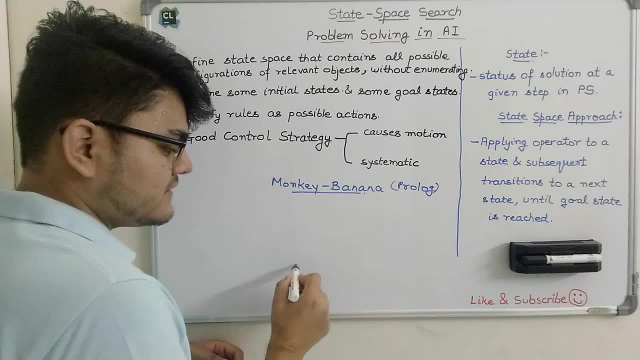 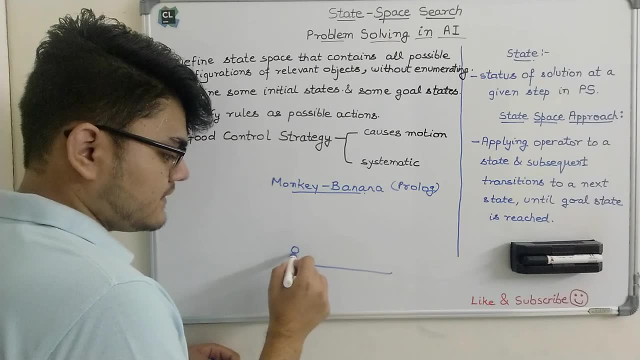 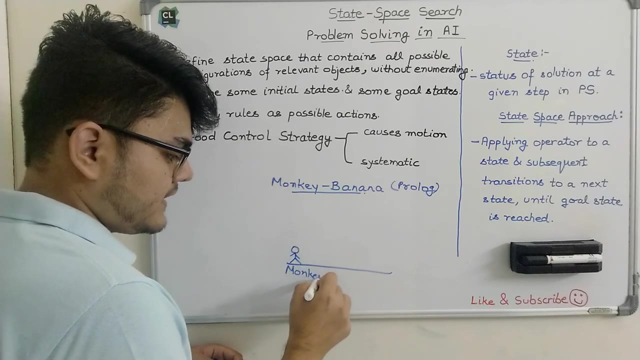 So now let's understand what the problem is. The problem is very simple. We have a monkey here, right? Let's say this is a monkey, Let's assume that this is a monkey, right, And we have some stacks here. 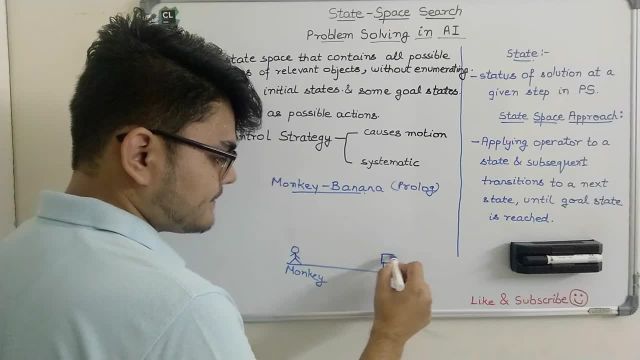 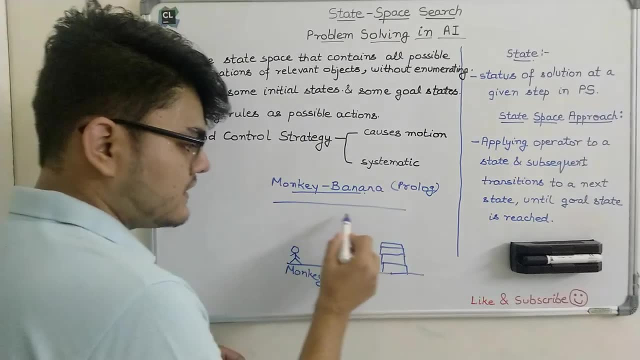 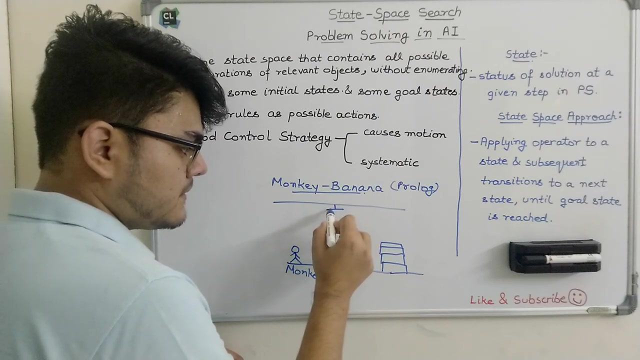 or I can say there are some blocks here, Let's say there are three or maybe four blocks. And on the roof let's say this is the roof and this is the ground. So on the roof there are bananas, right. 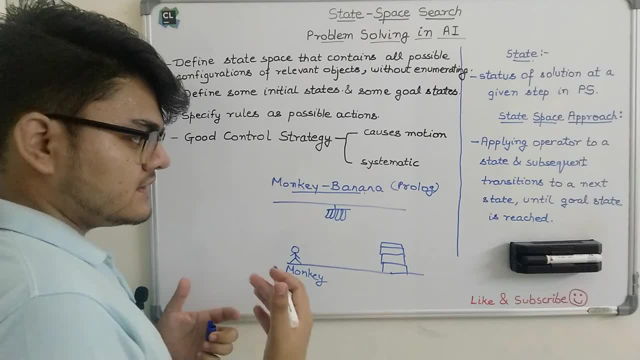 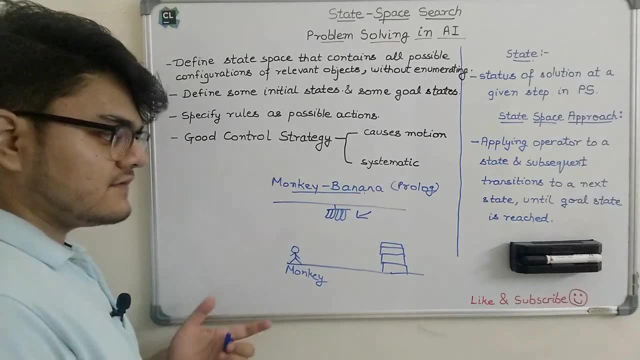 So now the problem is that we want to make sure that this monkey- whether this monkey can get these bananas or not- This is a very simple problem for humans to solve. First of all, if you will give this problem to a human, 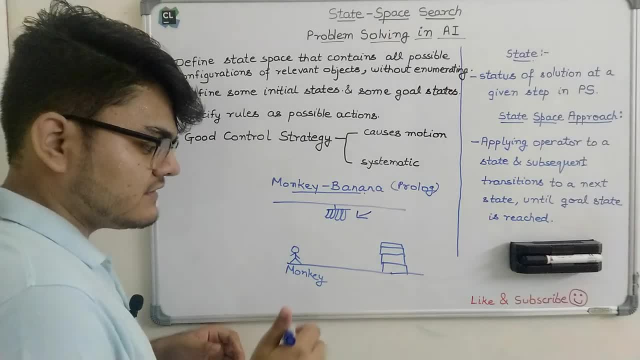 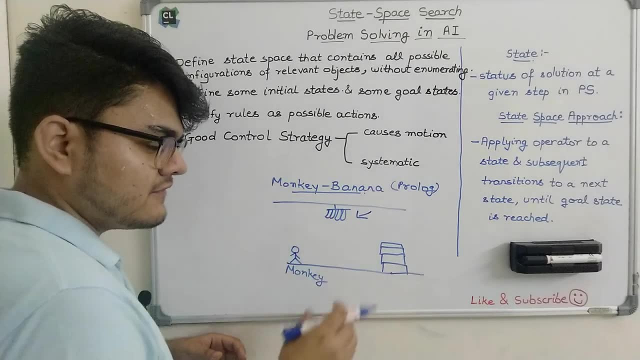 he will basically ask a few questions. For example, he will ask whether the monkey will be able to make sure that these stacks get aligned here, whether the monkey is intelligent, whether the monkey is intelligent enough to understand that he will have to move this or not. right, 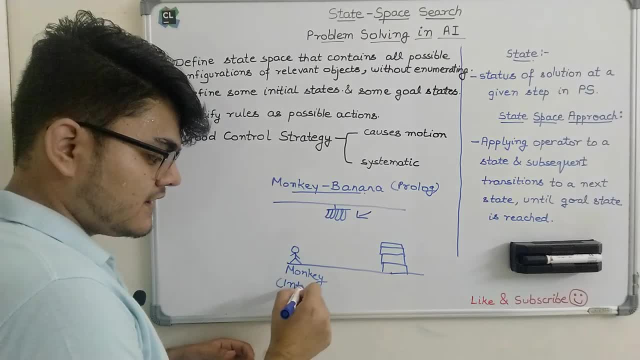 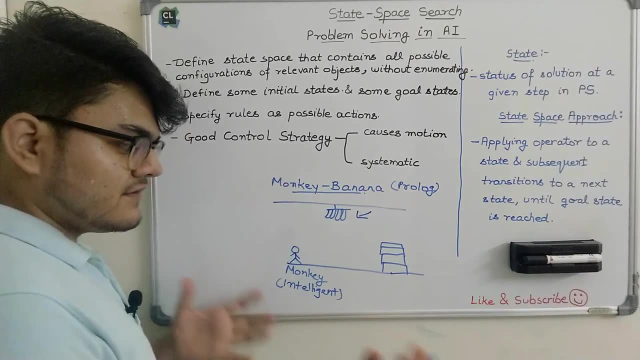 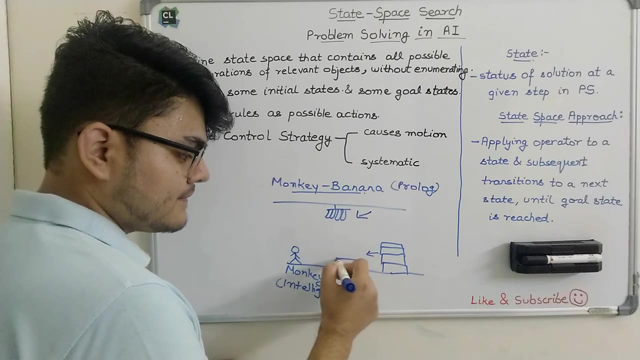 So the first question that a human will ask, that if the monkey is intelligent or not, Let's say, it is given that the monkey is intelligent and he can move these stacks. Now let's suppose he moves these stacks here. Now the second question that will come into your mind: 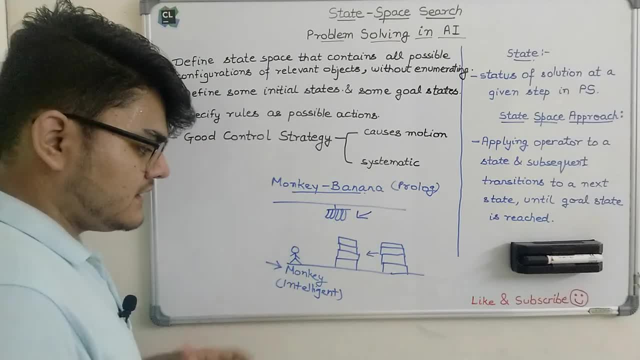 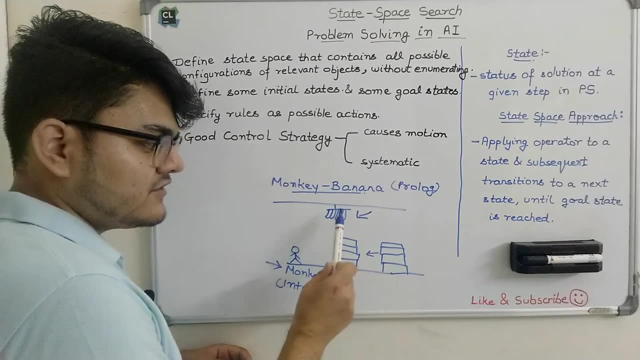 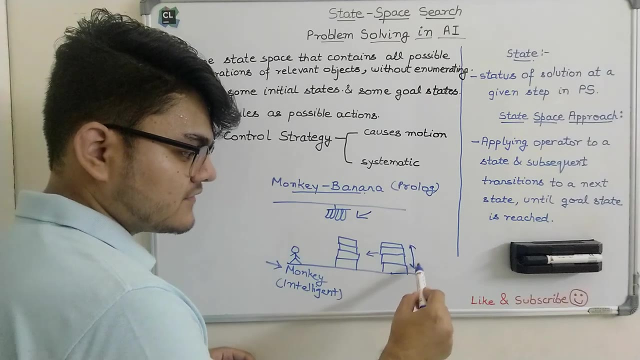 that will come into the mind of monkey- sorry, in your mind, because we are solving the problem- is whether the monkey will be able to reach the bananas on the roof, whether the height of the stack is enough to reach the bananas or not. right? 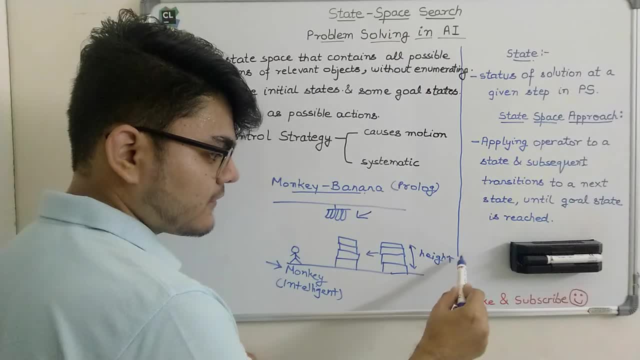 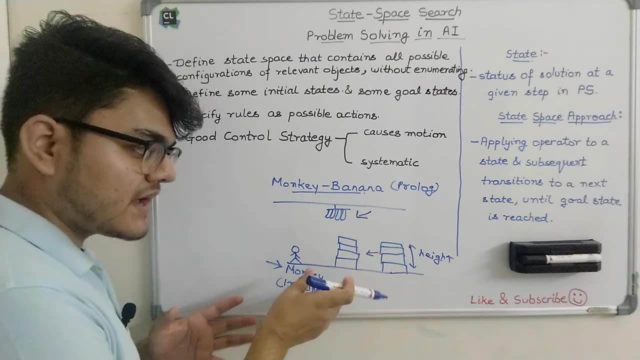 So we will have to understand whether the height is enough or not. Now let's say I've given this, that the given stacks, the monkey is intelligent enough to stack them up and he will also be able to reach the bananas because the height is. 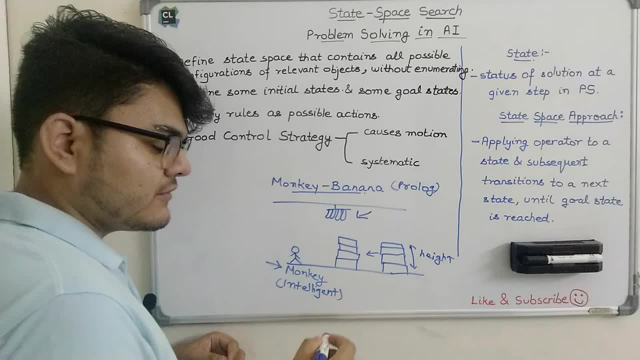 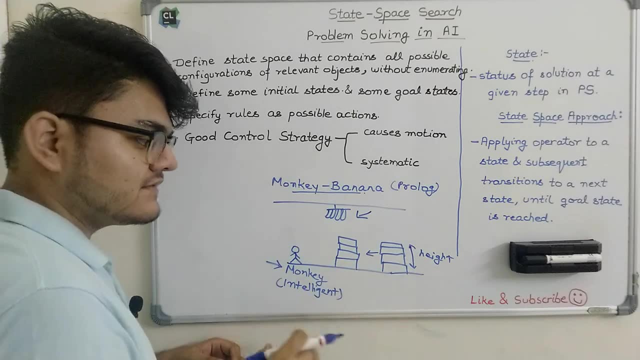 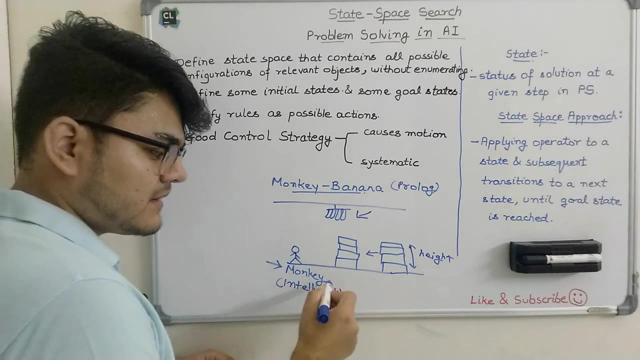 sufficient. So then, I ask you a very simple question: Given these things, that the height is there, we have these stacks. the monkey is intelligent enough to get these stacks lined up. Now I'm going to ask you a very simple question: will the monkey be able to grab these bananas or not? 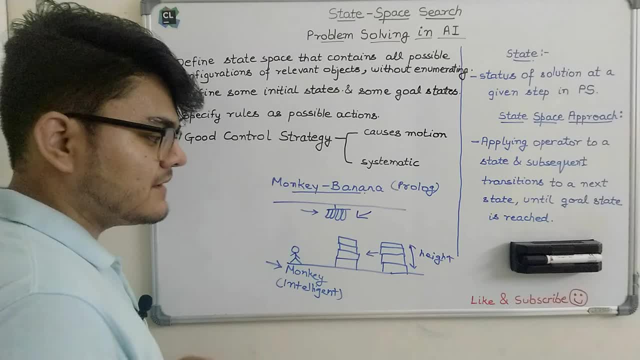 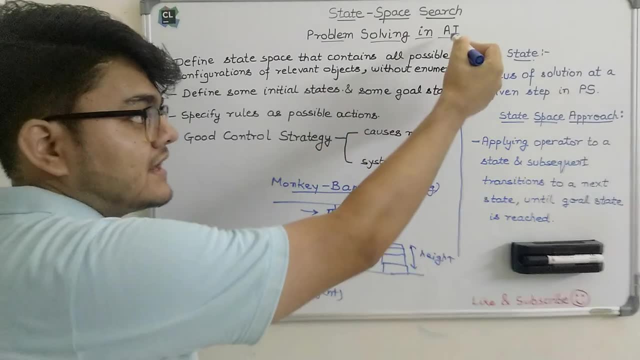 Now you will say it is a very simple answer. Yes, the monkey will be able to reach the bananas very simply, But just think of this problem as as an AI agent who is solving this For an AI agent. we will have to specify all the things. 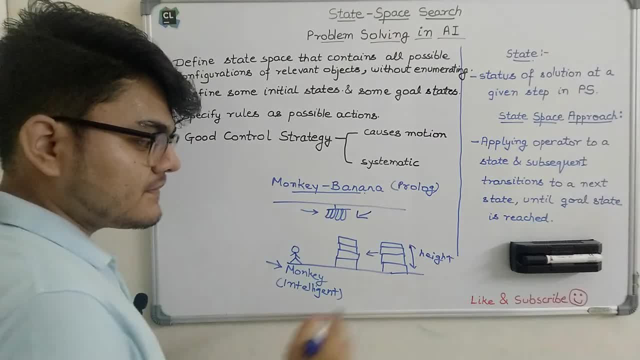 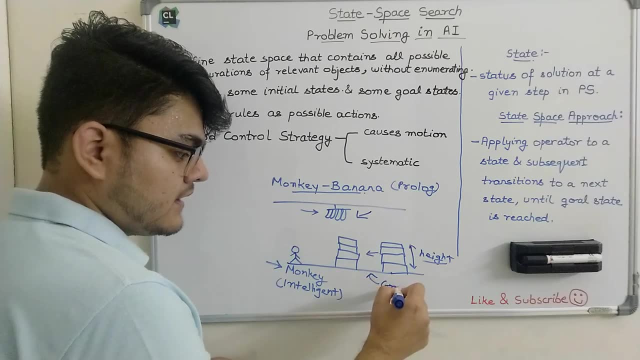 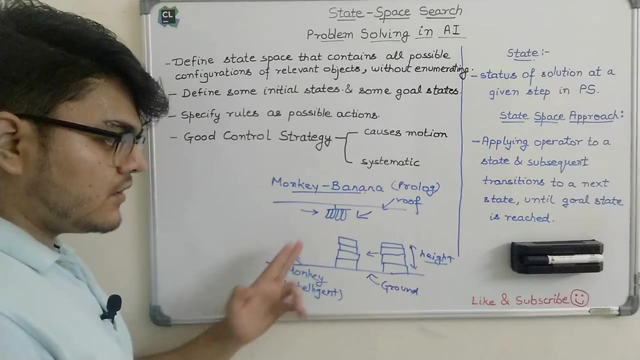 which are necessary for the monkey to grab the bananas. We will have to specify the height, we will have to specify the environment which is the ground, right With then roof, and that all things. Now you can see that the goal. 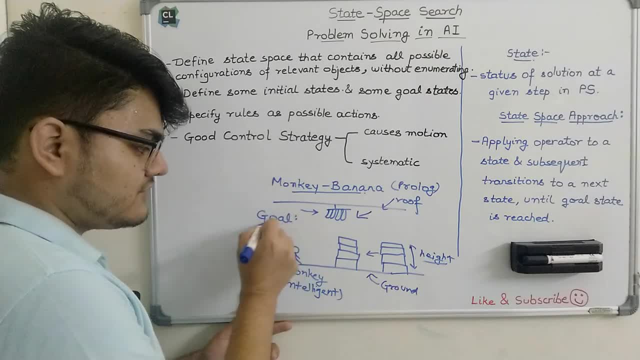 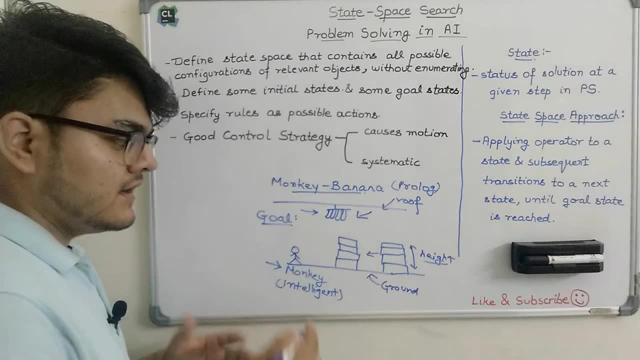 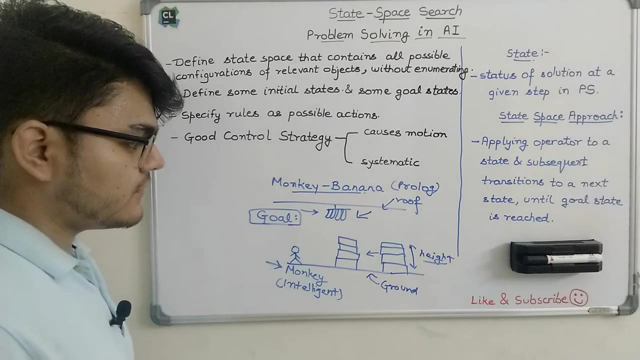 which is to reach the bananas right. the whole problem is that, whether the monkey will be able to grab the bananas or not, right? so the goal of this problem is to reach that monkey will be able to reach the bananas or not. 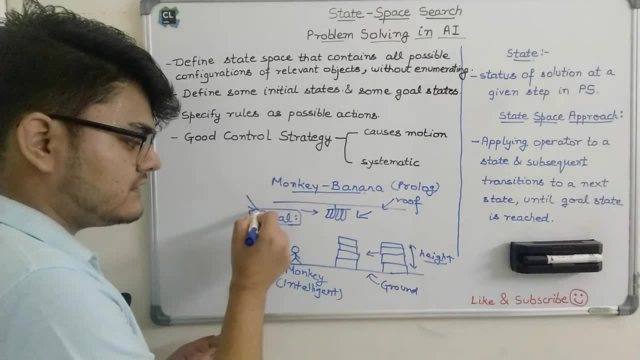 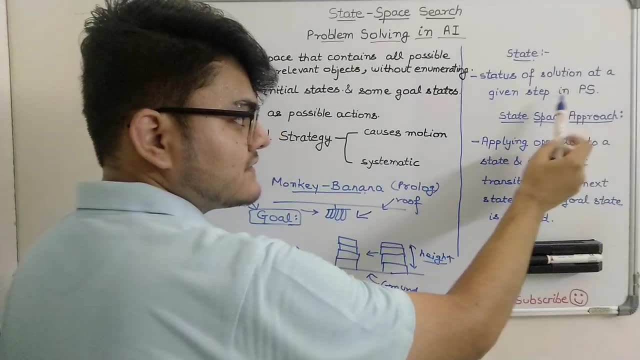 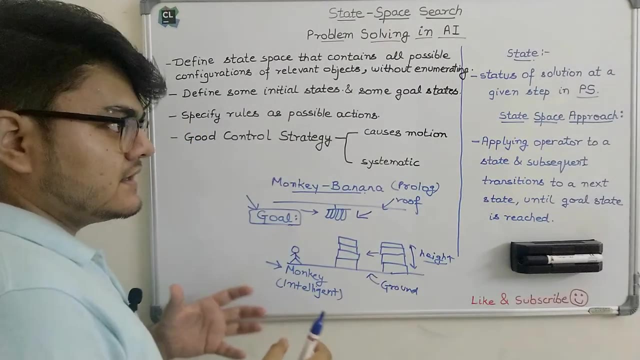 Now remember, in all the problems there are some goal states where we define a state as a status of solution at a given step in PS P. S means problem solving right, So it is a status of solution. it means that let's say, in this situation, in this very 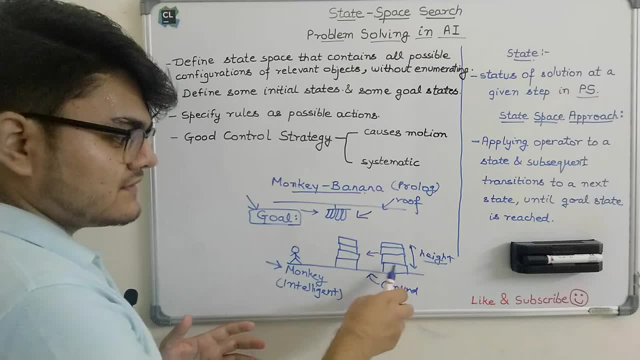 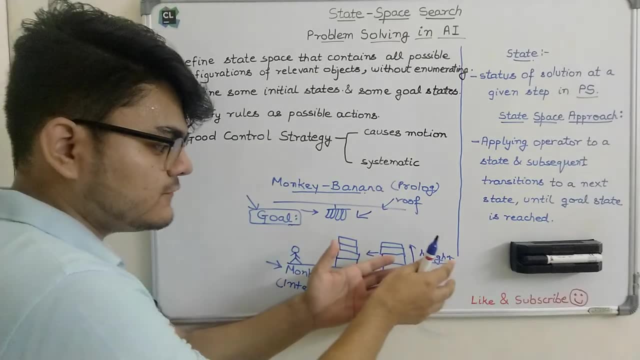 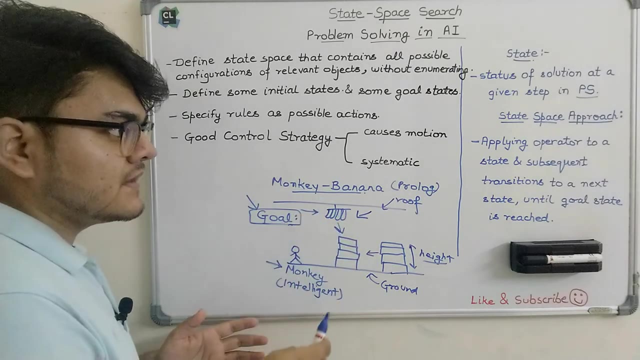 simple example. initial state was that the stacks were there and this was the bananas, and this is the monkey. in the next state, the monkey moves these stack and aligns it in front of these bananas so that he can read there. so it is actually a part of the solution, right? so these, all these, are the part of the. 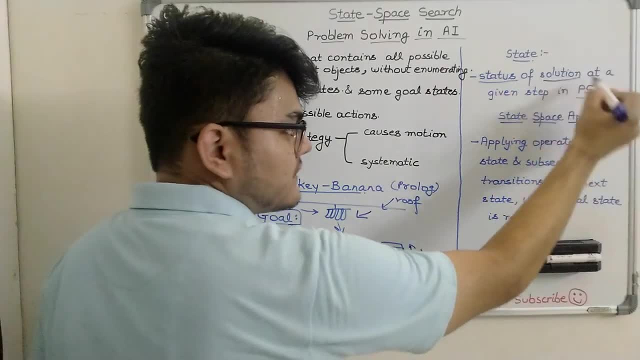 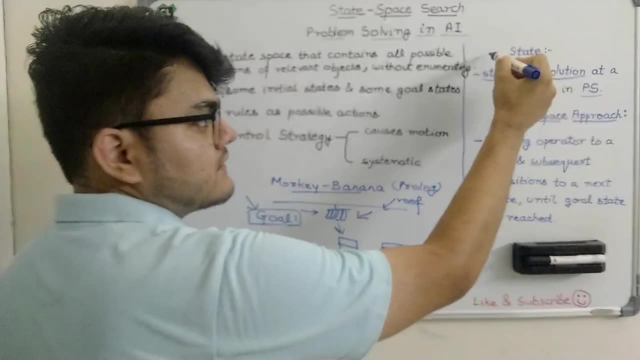 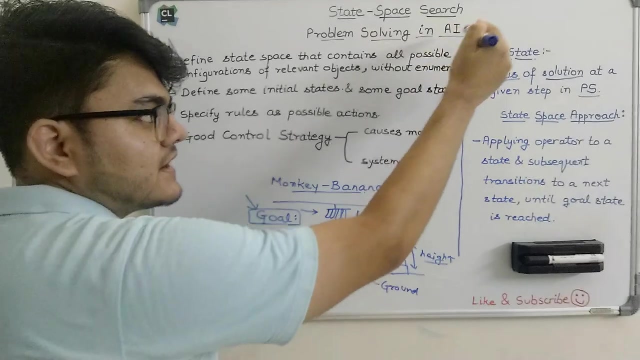 solution. so part means it is a status of the solution at a given step in problem solving right. so what we try to do is: first we are going to specify the states of the problem that we are introducing. we will have to specify it to the artificial intelligence intelligence agent. we will have to specify the states. 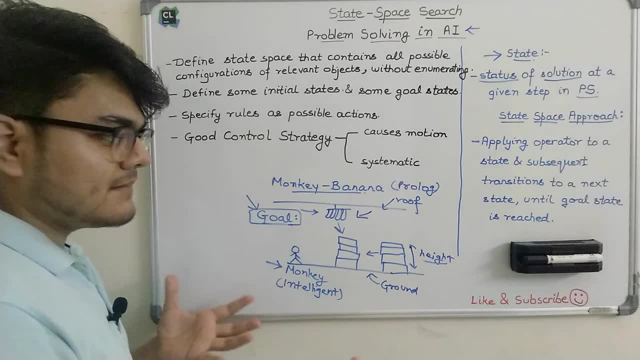 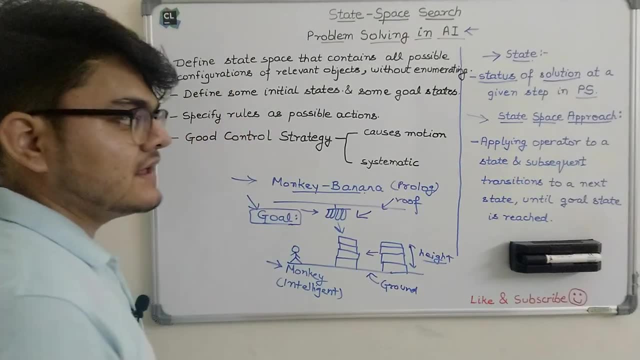 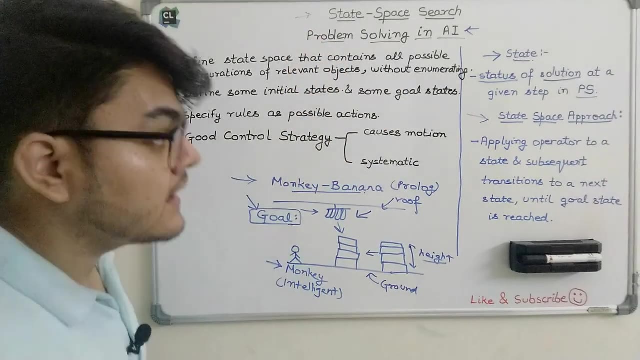 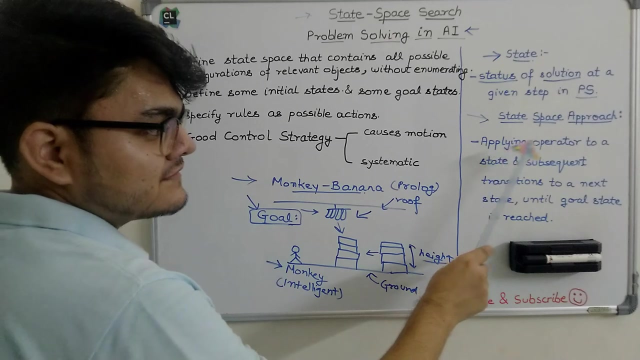 that are involved in the problem, involved in this problem. right, The problem can be anything. I'm just giving this very simple general example. Now let's take a look at what exactly is state space approach? Now, this is the main heading you can see here. Now, what is state space approach? State space approach is just. 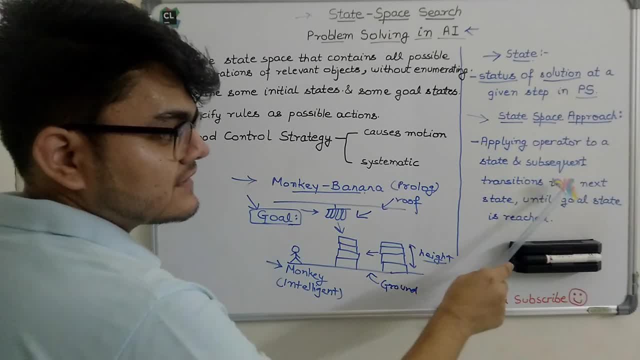 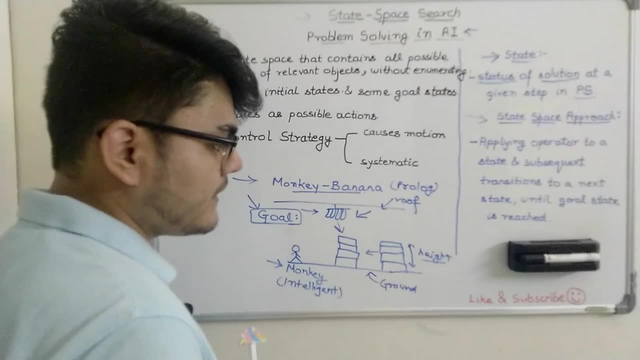 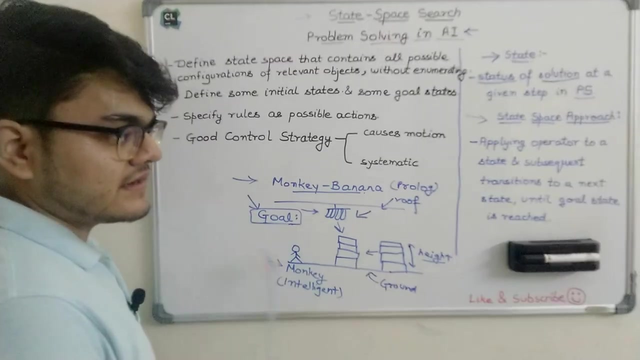 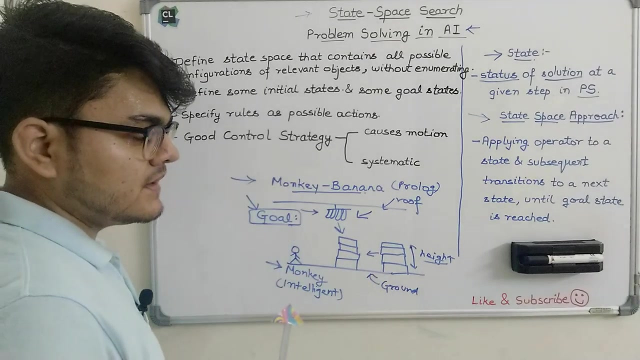 applying operator to a state and subsequent transitions to a next state until and unless the goal state is reached right. So the main objective of any particular problem is to reach the goal state right. So how will an AI agent reach the goal? The answer is that there are some. 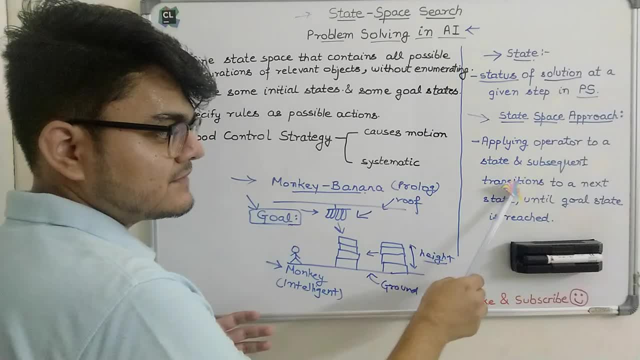 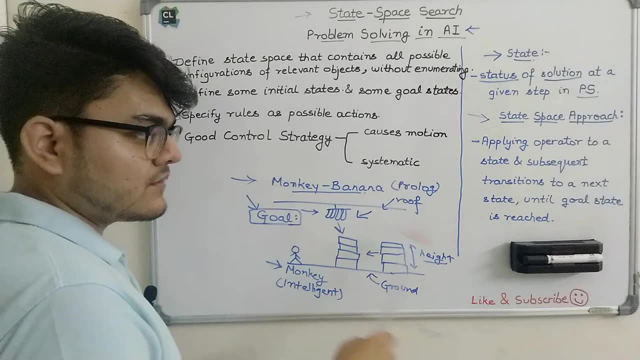 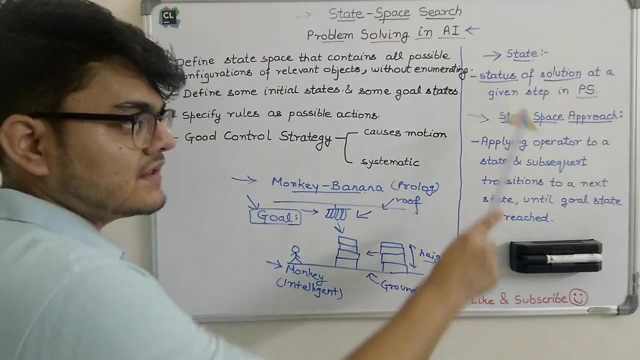 states in between, And these we call as the subsequent transitions, We will have to move from one state to the other state and we will go on like this until and unless the goal state is reached. This is known as state space approach. State space means state means that all the states that will contribute to the 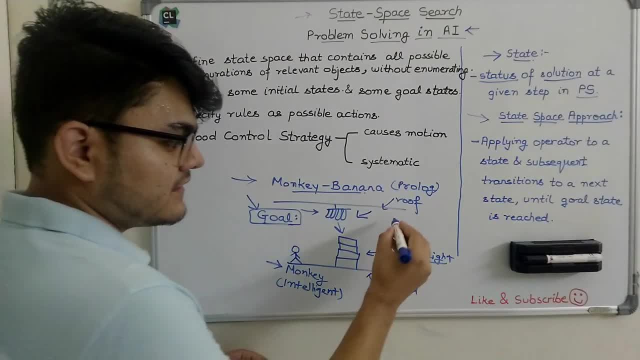 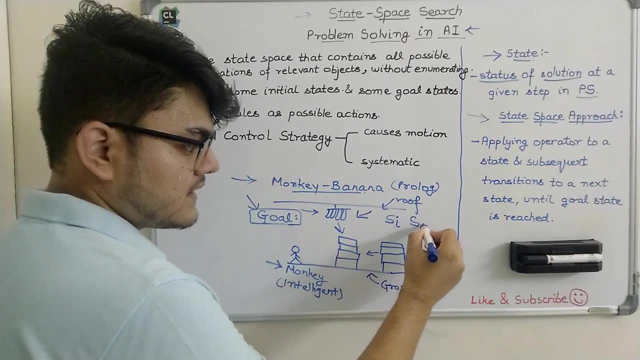 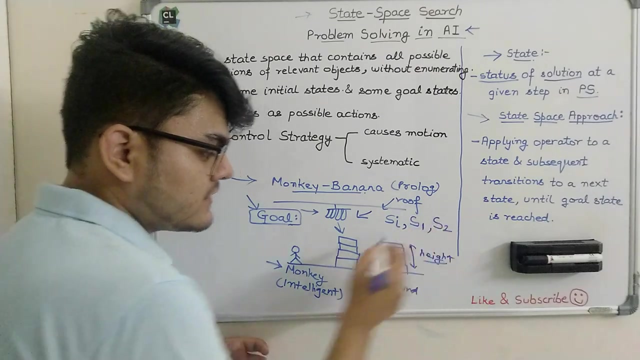 solution, right? So let's suppose the initial state, let's say SI, was when the stacks were hit. Then we say there is S1,, which is another state when the monkey moves the stack here. Let's say there is another state to where the monkey is climbing, has climbed these stacks. right Then? 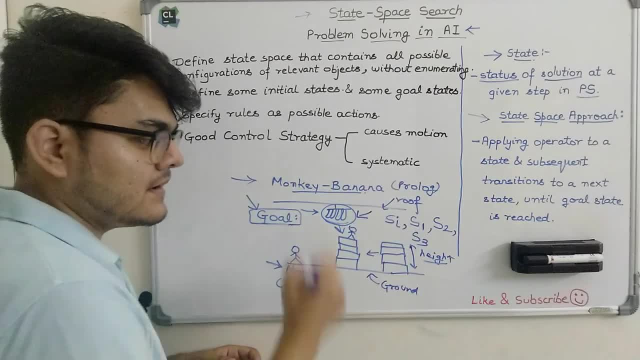 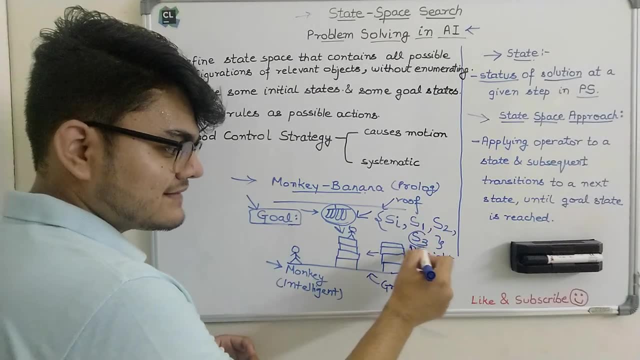 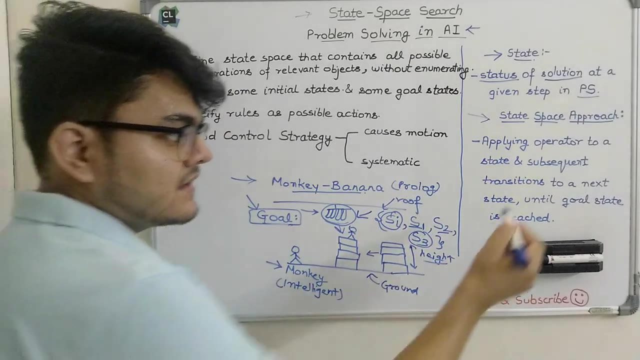 let's say the third stage is the final stage, when he has grabbed the bananas. All these states are contributing to the solution. We know that the goal state is S3.. Initial state is SI. So the goal state is SI And these states, S1 and S2, are also necessary. These are known as subsequent. 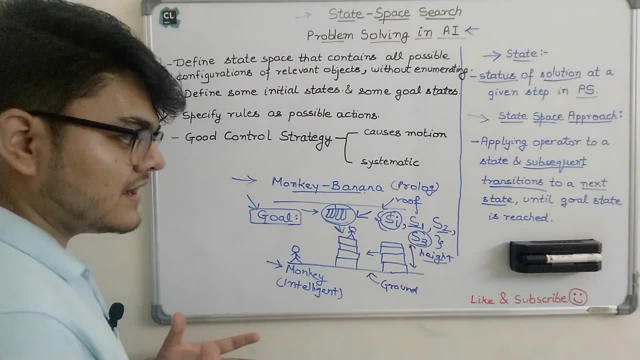 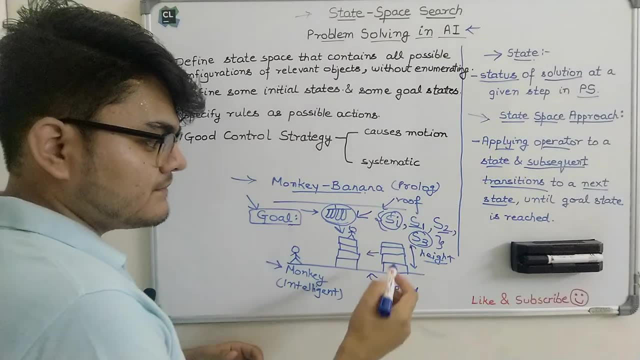 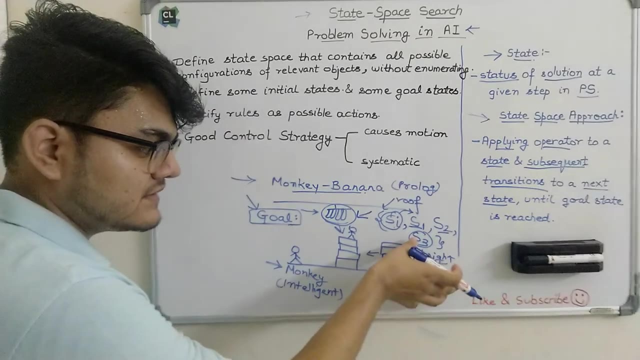 transitions to a next state. This is the meaning right. So applying operator to a state means that we are actually doing some operation. You can see, to reach from initial state to S1, I will actually have to move, The monkey will have to move these stacks here. right, This is the main use of 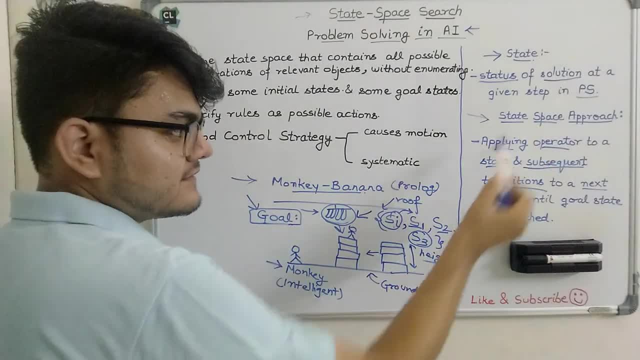 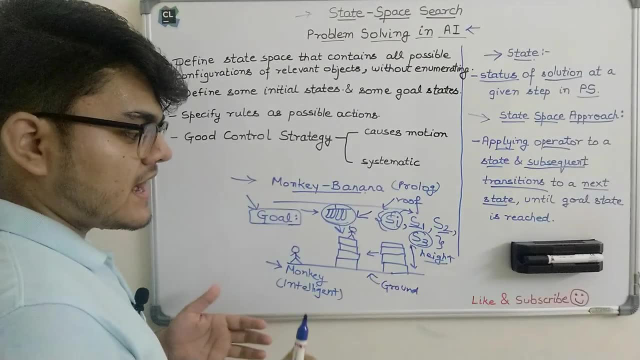 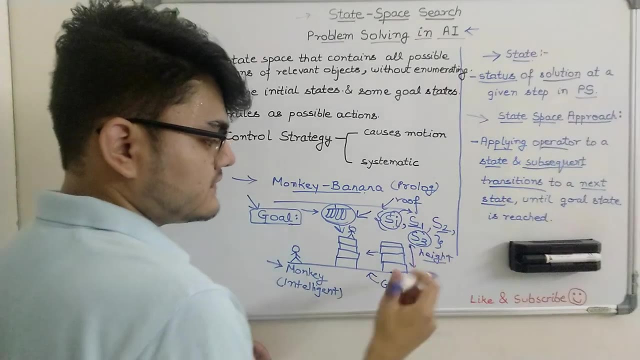 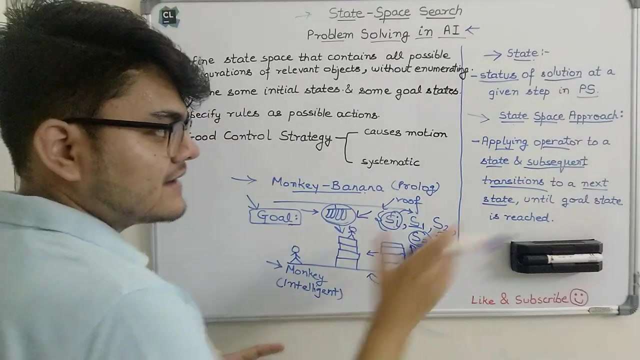 applying an operator. So states are the states. you can see now here from the problem that we will have some states and those states must contribute to the solution. right Now these states are, you can see, this is a set, So that's why we call them state space, right? So this is the whole state space And this is the 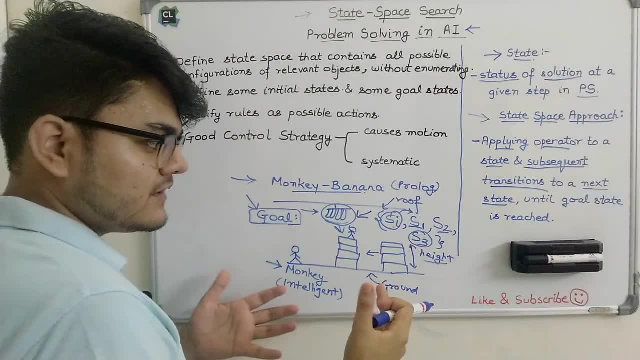 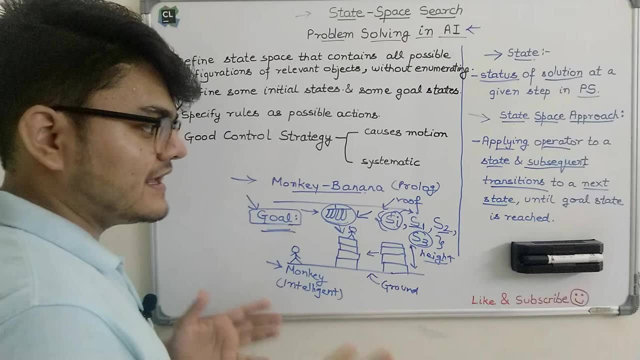 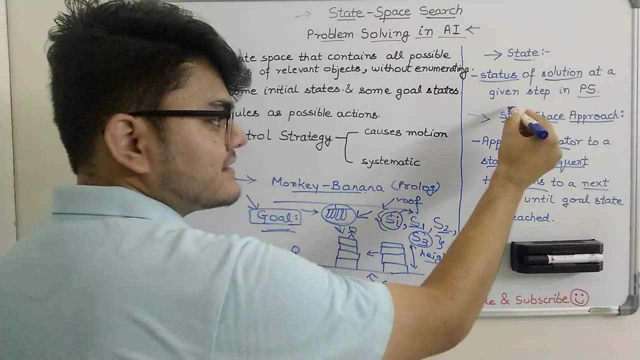 approach that we are going to use, or the AI agent will use, to actually reach the goal state right. The purpose of the AI agent is to solve the problem, just like humans, So for that we will have to supply the agent with all the states that are available, or we can just say all the state space We will. 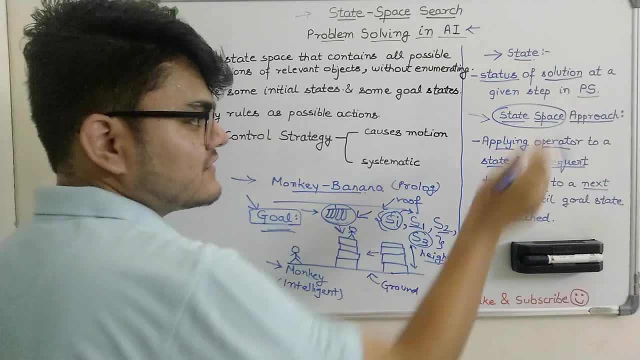 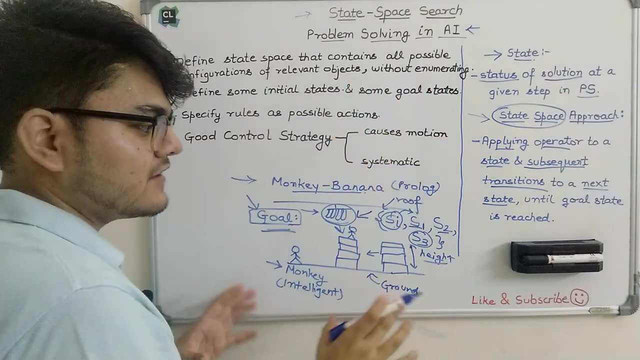 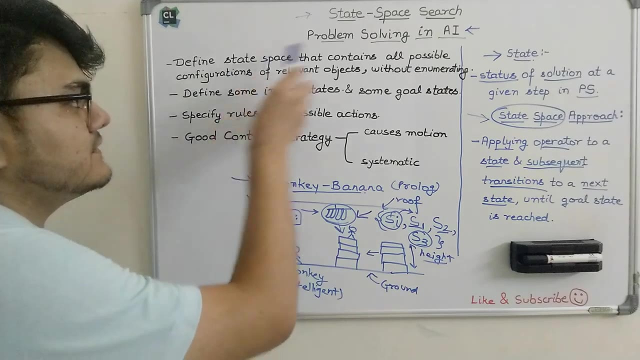 provide it with the state space right. So this is basic definition of state and state space approach. Now let's see a general way to represent any problem in artificial intelligence using this state space search algorithm. right, If you look at this picture, we have the state space search problem, right? So this approach. you can see that here I have. 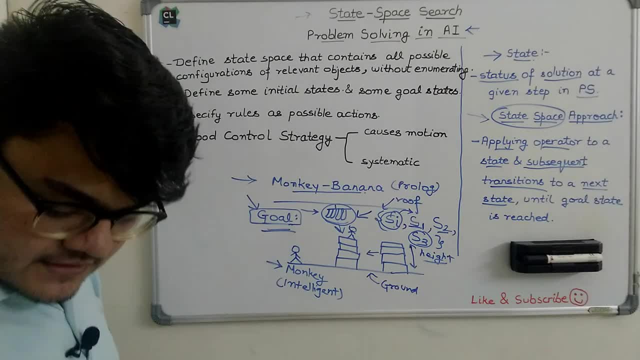 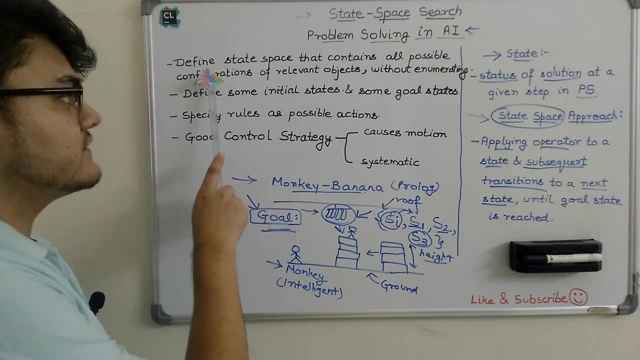 written some four steps here which you will use, or which you can use, to actually represent a problem as a state space search problem, right? So let's start from the first one: Define state space, which is all the states that contains all the possible configurations of relevant objects. 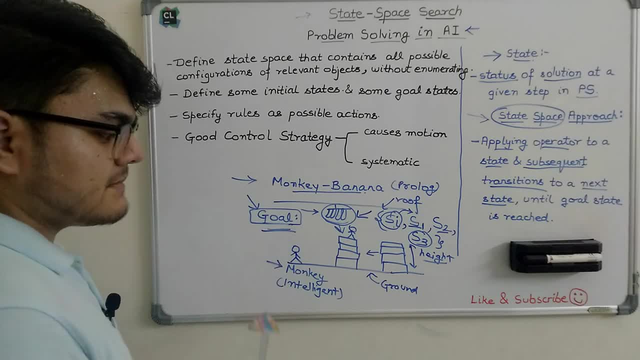 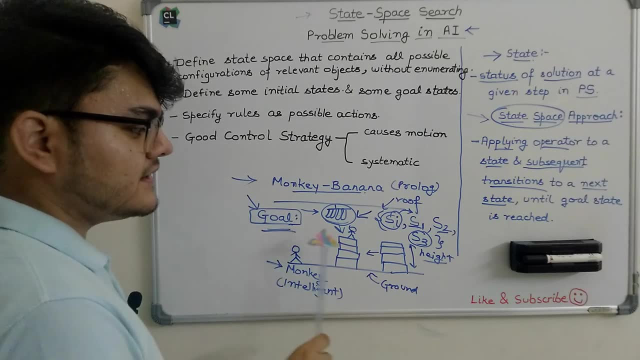 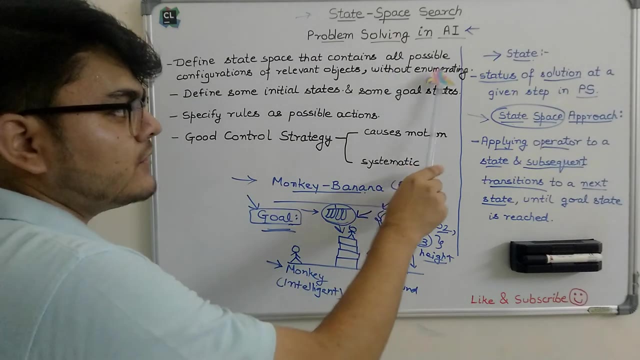 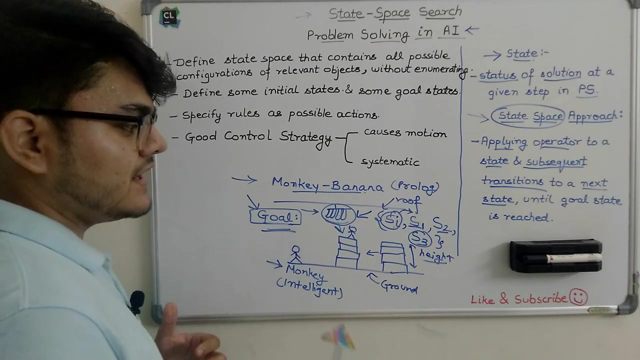 From this example: objects, stacks, bananas, monkey ground roof. all these are relevant why? because all these are needed, because if we will miss any one of these, the monkey will not be able to reach the bananas without enumerating. enumerating means we are not actually stuck on one single transition right. 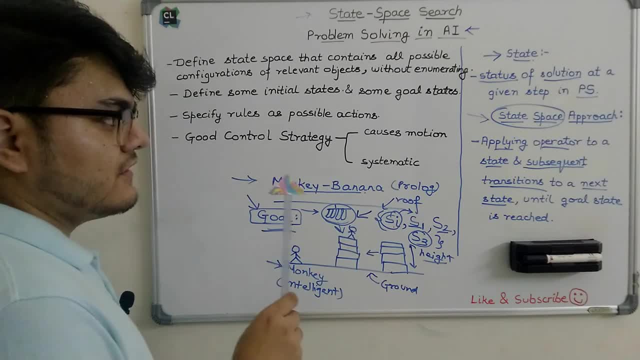 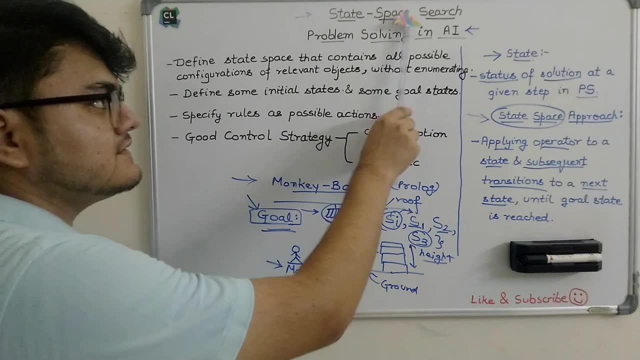 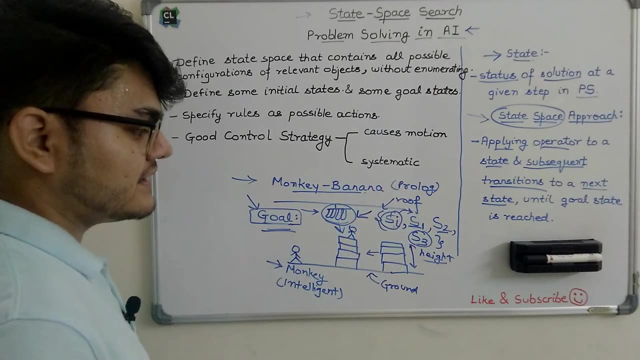 we are not enumerating on a single state. after every state we are moving to some other state. the second step in the state space approach is that you should, you must define initial states and some goal states. initial states: you can see, this is the si, is the initial state of the problem. 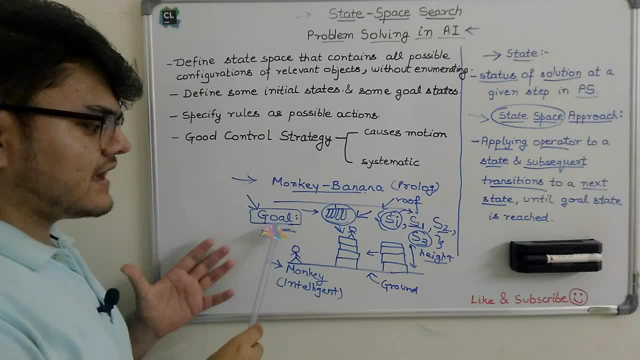 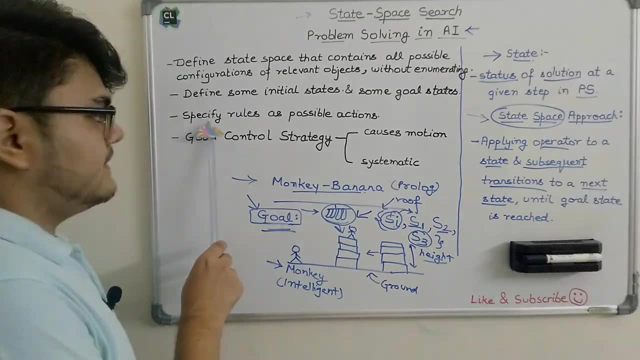 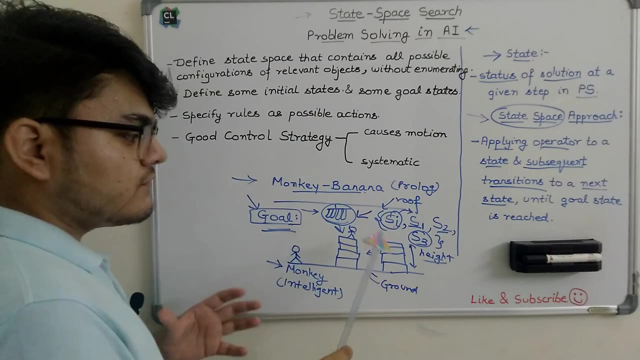 and you will have to specify the goal state. sometimes they can. there can be multiple initial states in a problem and multiple goal states also. next is to specify rules as possible actions right, very important step: to move from one state to another. why we are moving from one state to another? the answer: 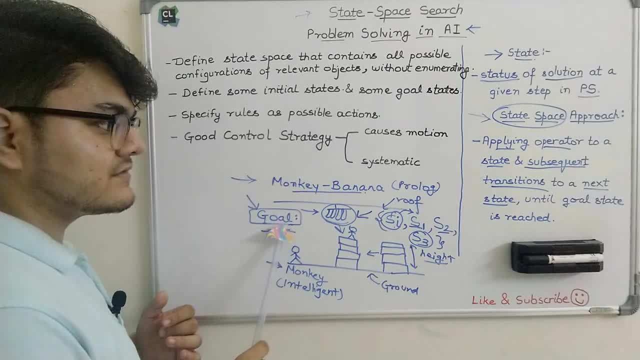 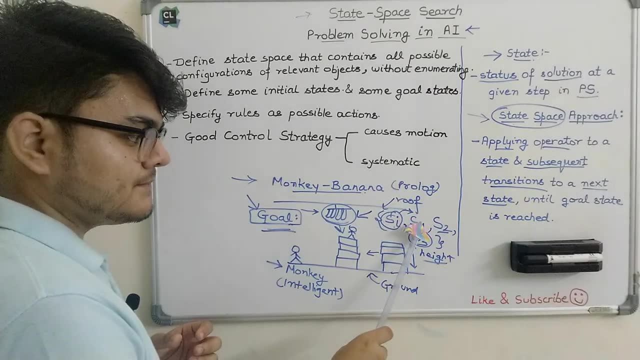 is simple: because we want the solution, we want to reach the goal state right until goal state is reached. so in that case, from one state to the other other relevant state, we need to perform something like this. so in that case, we need to perform something like this. so in that case, 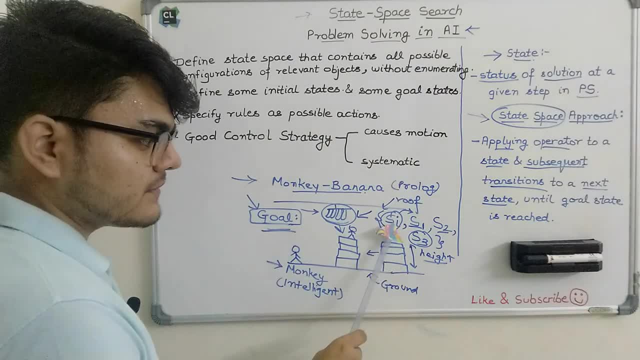 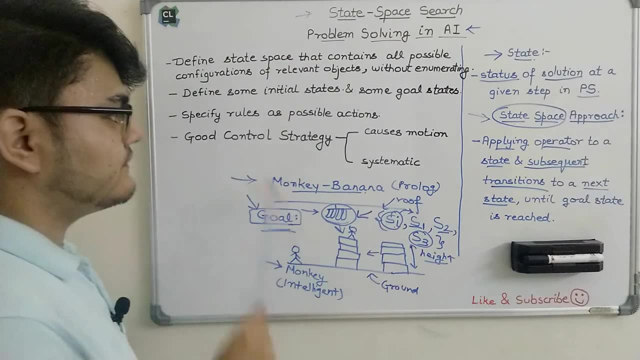 some action right. for example, if i want to move from state si to s1, i will have to move the stacks here. so specify rules as possible actions. we will have to specify these rules. so this is the basic and the general way to represent any problem in artificial intelligence as the state space. 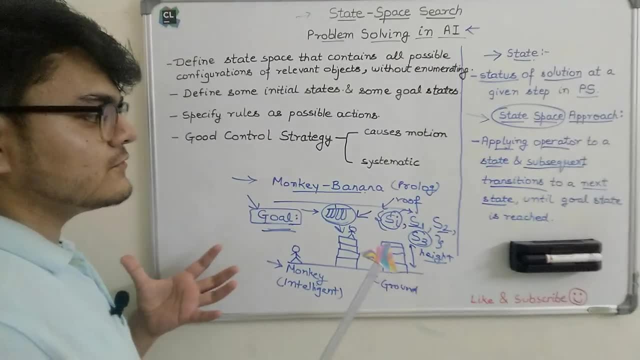 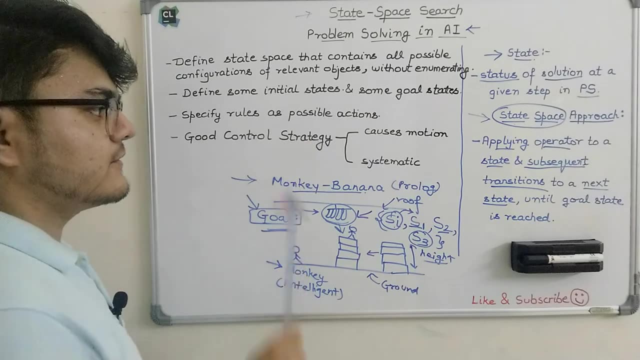 problem right. it is a general approach to solve the problems by artificial intelligent agent. the last step in the state space approach is to specify rules as possible actions. we will have to specify these rules at the end of the step. so first step is this. last step which, in the case, 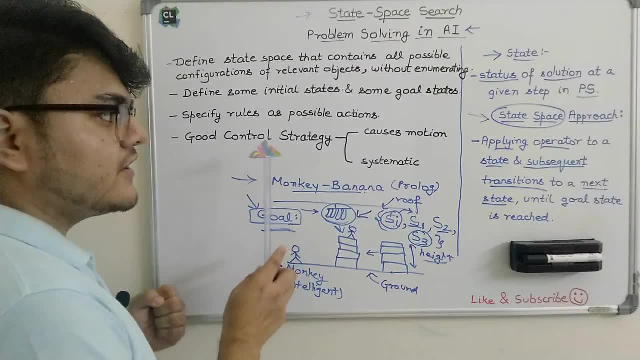 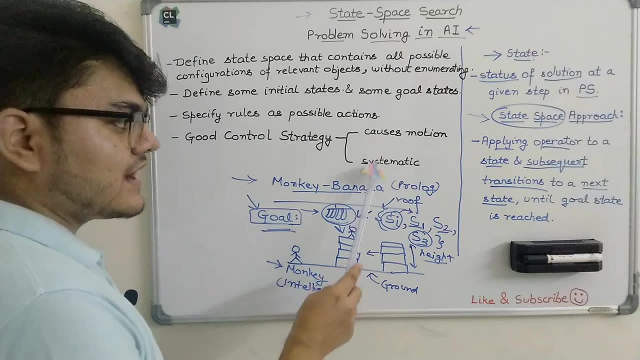 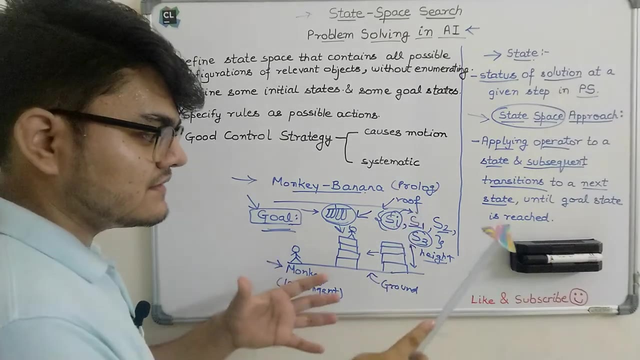 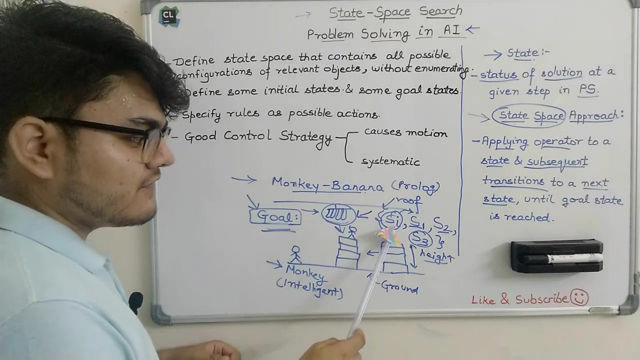 of fresh throwing Lord's shver's. shver's is the step for對ər. you need to define several objects in the table by highlighting one object and then going through these multiple art которая. this is, looking for hand the two structures, you can see that if I try to move from SI to S1, which is from initial state to the S1 state, you 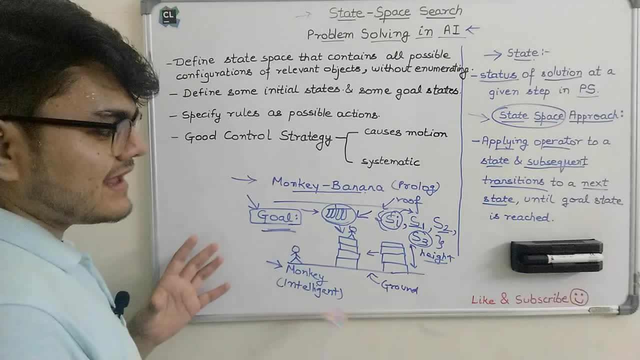 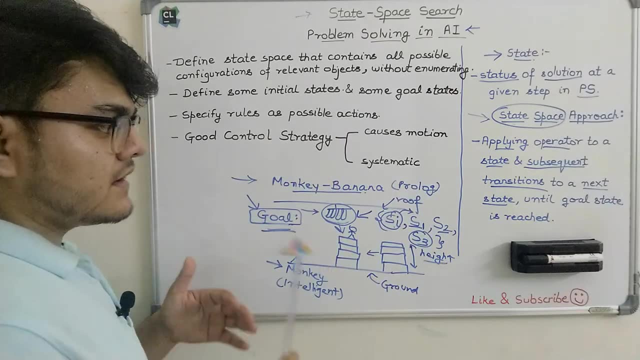 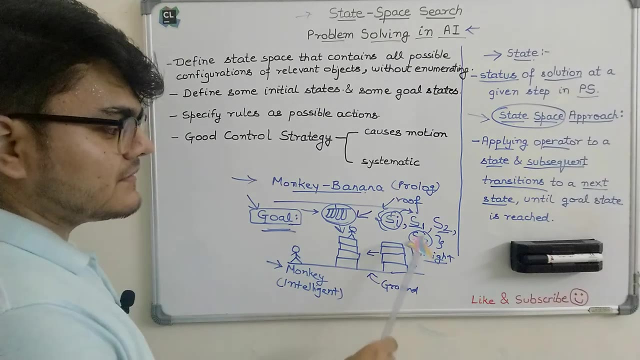 can see the motion is of these stacks. I'm just giving this as an example. you can use this as an example to understand what is going on here, and there are a lot of problems that we will discuss, like water jug problem and n queens problem. there are a lot of problems that we will. 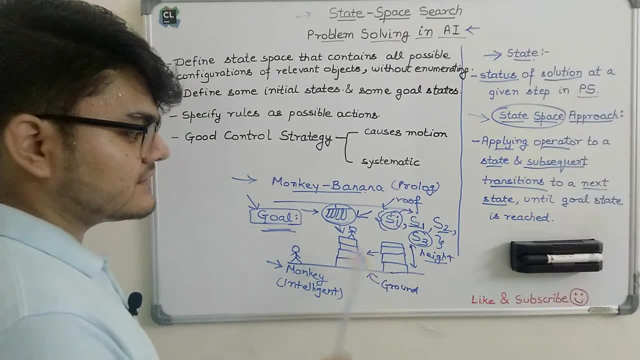 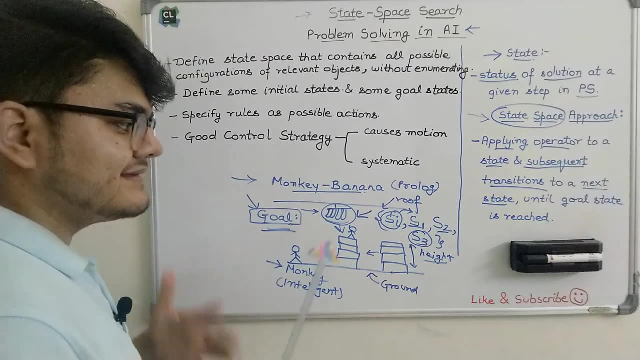 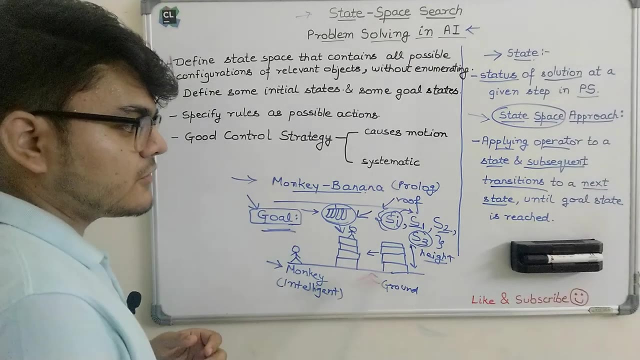 discuss, and that's why we are studying this simple example, because I find this very interesting. I've also written the prologue program, so I basically know how this, how these AI programs, are written right. so this is a very good problem to pick up right. next one is the systematic, systematic means. 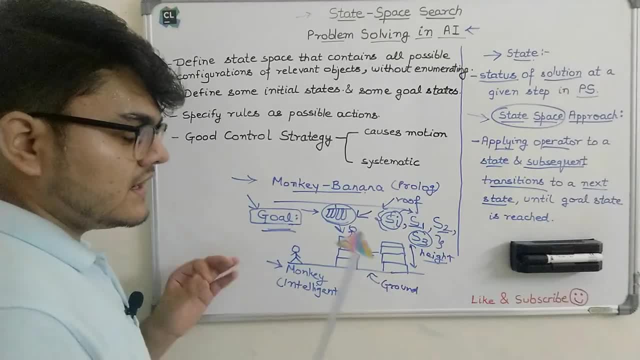 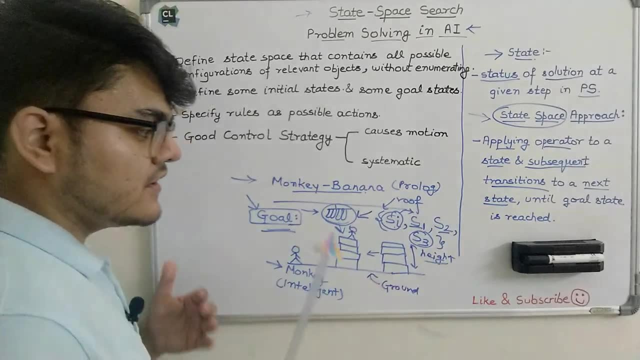 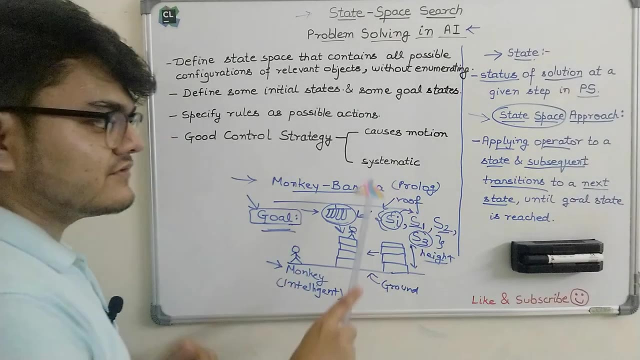 that if you are moving from one state to the other state, it is necessary that this state s1, s2- must be some relevant state and using these states, you are able to reach the goal state. if you are not reaching the goal state, these states are irrelevant, right? so there should. 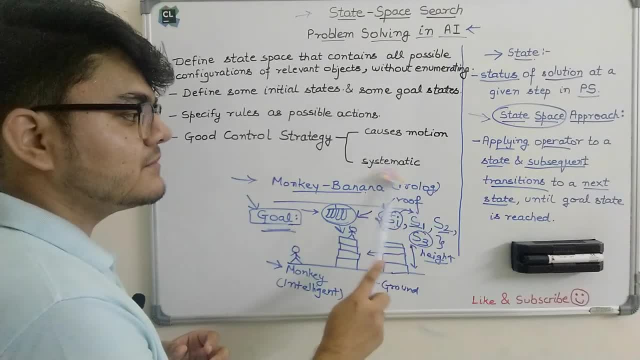 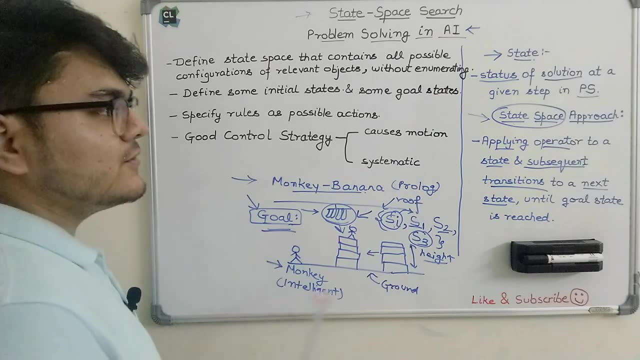 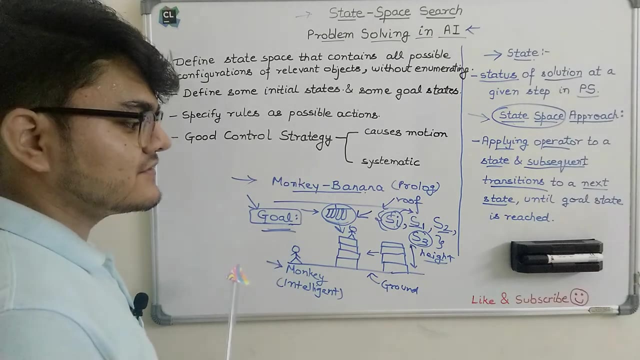 be some systematic movement. movement should be there, but it should be also systematic, and these are the two strategies to actually control this. so in this way we can do problem-solving in the air using state space search. so that's all for this tutorial, if you have liked this tutorial.